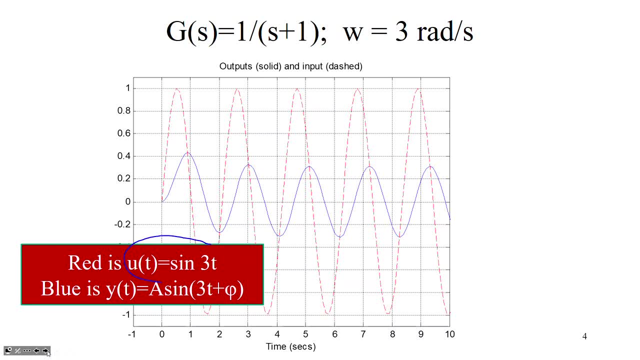 The input signal is sine of three t, And that's given by this red line here, And the output signal is a sine three t plus phi, And that's given by this blue signal here. Now, what I've done is I've ignored the transients. 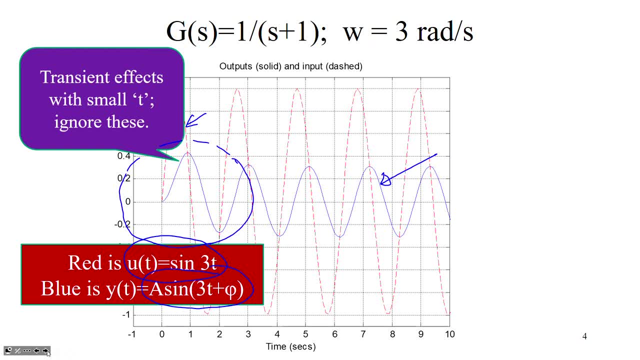 If you look carefully, you'll see that during the transients we've not settled just to a sinusoid. There's some other stuff going on, So let's ignore that. If we do that, what you'll see is, asymptotically, we're going to get a fixed phase and gain. 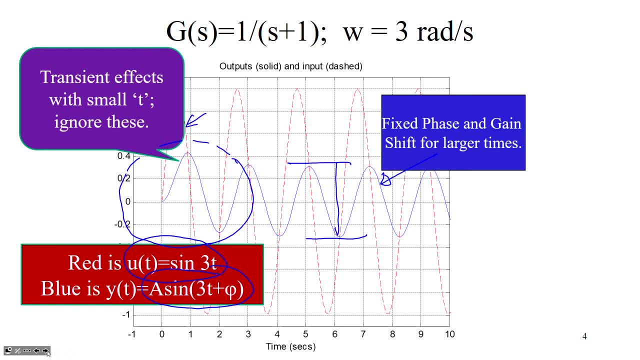 All right, We can actually work out what the gain is. So a that distance, there is going to be two. a, All right. And we can also see that there's a phase shift: There's the peak for the input and there's the peak for the output. 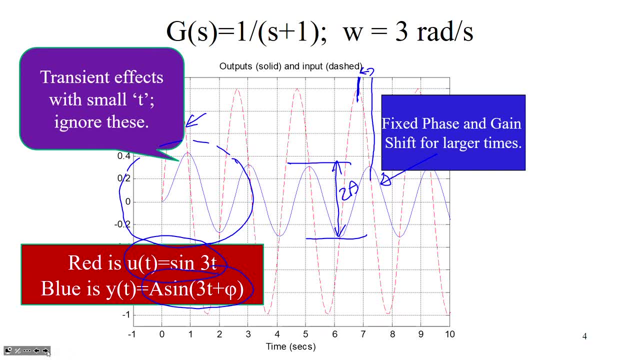 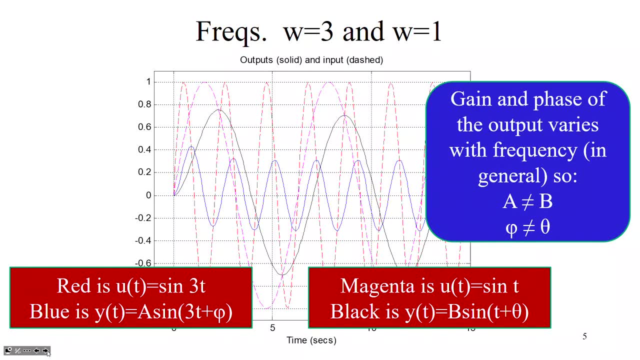 And you'll see there's a difference in phase between those two signals. Now what happens if we change the frequency? Now this picture looks quite busy, but if I do it slowly you'll see what's going on. So this red line here, OK, is this signal: u of t equals sine three t. 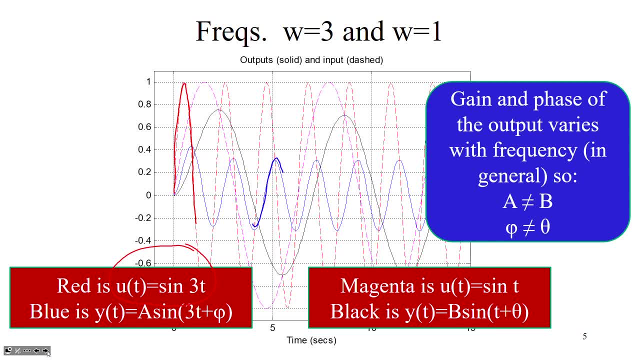 And that goes with this output line here, blue, You'll see they've got the same frequency. Now what do you notice? There's a particular gain and a particular phase for that output. Now what happens if I have a different input signal? 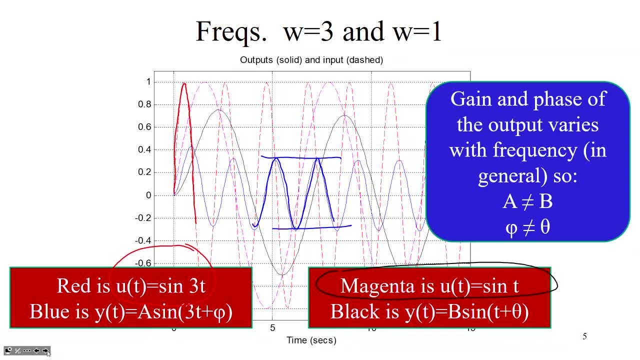 So the magenta curve is sine t. So if you follow that, you'll see it's also a sinusoid, but it's a much slower frequency sinusoid. So there it is. There's the magenta curve. My plot isn't perfect. And where's the corresponding output? 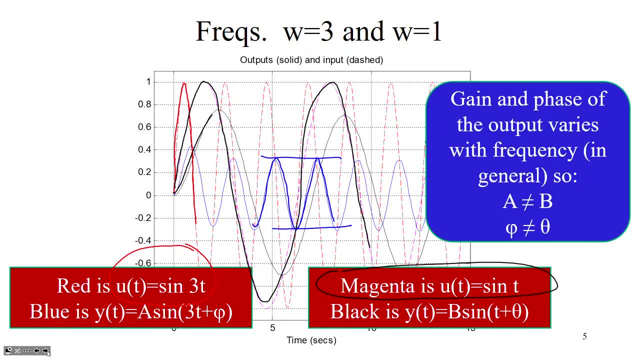 Well, it's in black And you'll see. here is the corresponding output. And what do you notice is interesting about this? Again, if you ignore transients, the amplitude is very, very different. So change the frequency and you get a different amplitude, which is what we've written here. 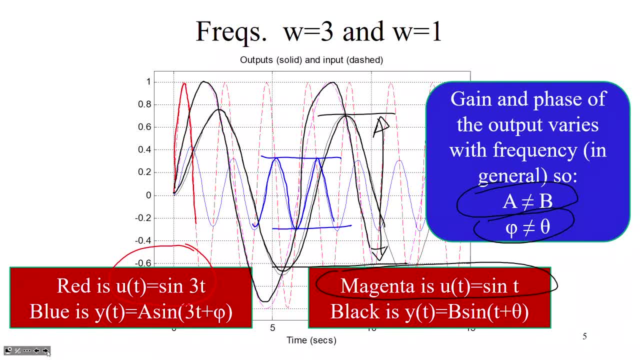 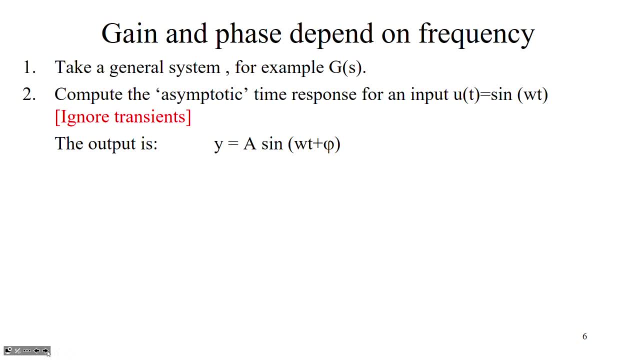 And if you look closely you'll see you also get a different phase. So if you take a general system G and you compute the asymptotic time response for some signal u equals sine omega t. the output is going to be a sine omega t plus phi. 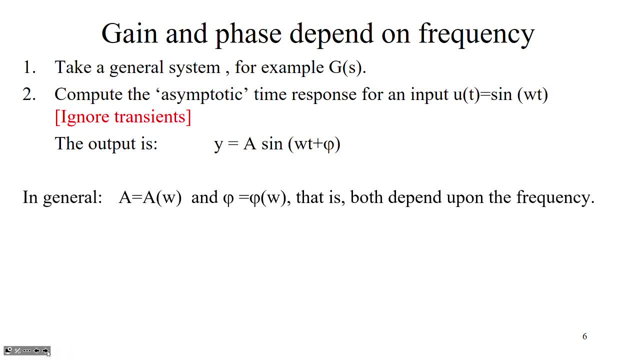 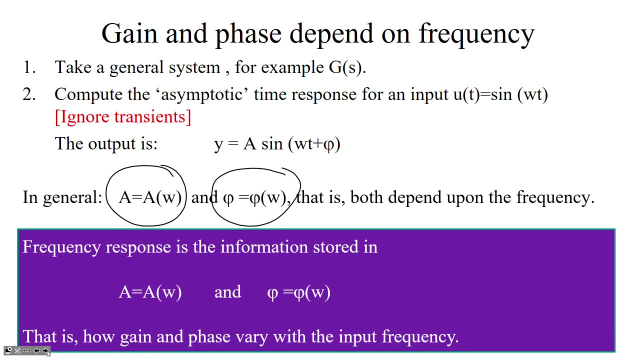 And, in general, you'll find that the amplitude a and the phase phi both depend upon frequency. So as you change frequency you get a different amplitude and a different phase. So what, then, is frequency response? Frequency response is simply the information stored. 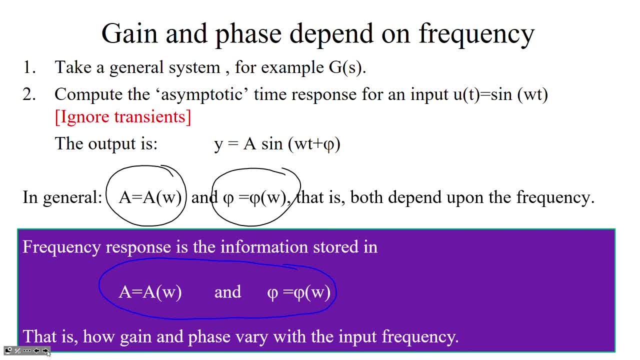 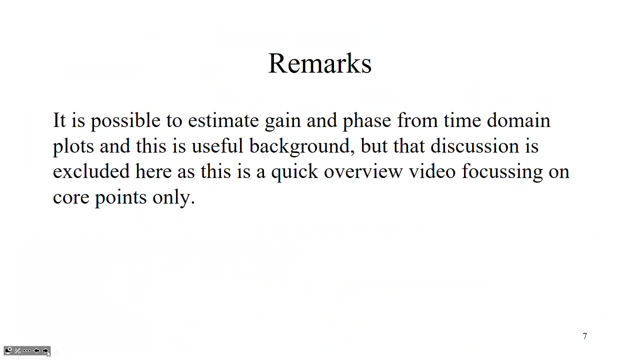 in these two variables, So a of omega and phi of omega. In other words, how do gain and phase vary as I change the frequency of the input to the system? Now it is possible to estimate the gain and phase from time. domain plots. 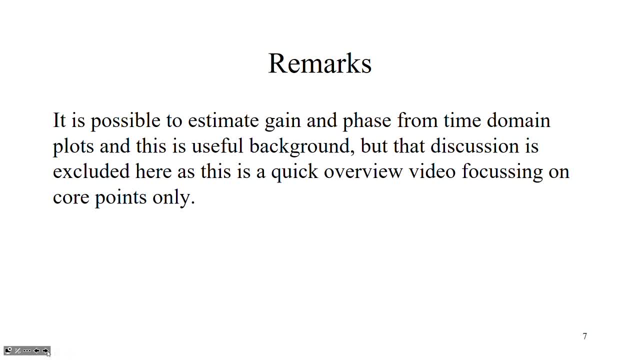 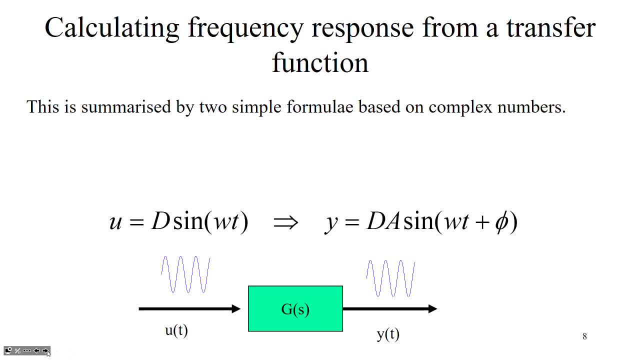 and this is useful background. But given this isn't a quick overview video, I'm not going to bother with that. You can do that in slower time if you like. What we need to focus on now is: how do we know that? How do we actually calculate the frequency response? 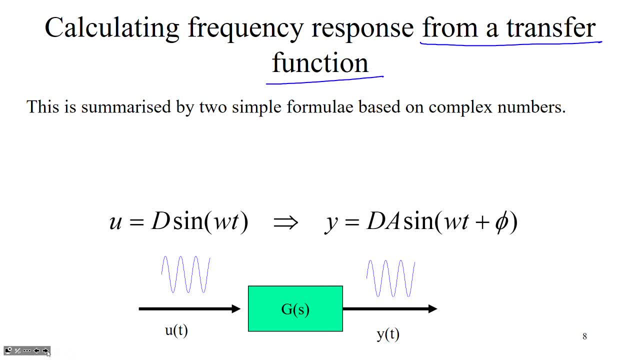 And here you'll see I'm going to say from a transfer function. So, if I know the transfer function of the system G of s, so we're focusing on linear systems- how can I work out what is this a and what is this phi? 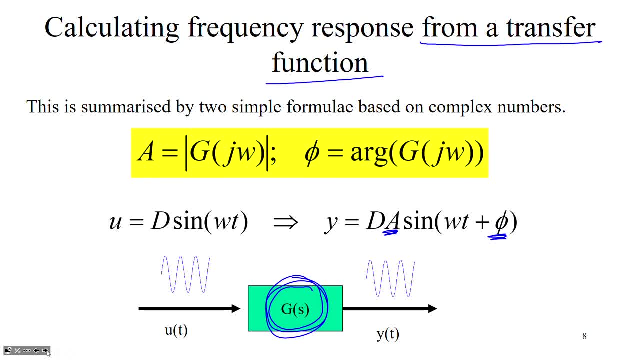 Well, it so happens that there are some very simple formula You can show that a is the modulus of G of j omega and phi is the argument of G of j omega. So you've got some very, very simple formula You can use to calculate the gain and the phase. 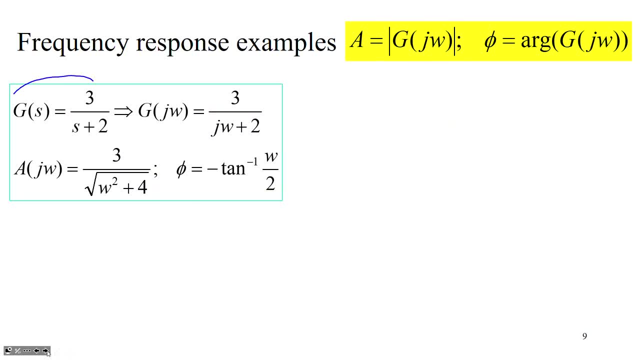 Let's give some examples, then. So we start with: G of s equals three over s plus two, And then what I'm doing is I'm simply replacing s by j omega, And you see, therefore I get three over j omega plus two. 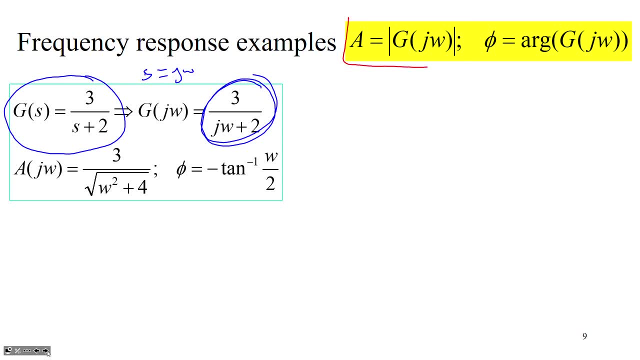 And then I look at my definitions which I put at the top here. So the gain is the modulus of G of j omega and the phase is the argument of G of j omega. And so you see, if I have a complex number three over j omega plus two, 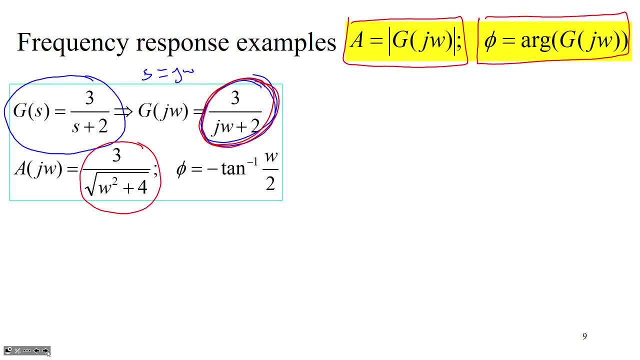 then the gain has got to be three over the square root of omega, squared plus four, And the phase is going to be tan to the minus one of omega over two. Now, assuming you know complex numbers, you probably think: yeah, that's straightforward. 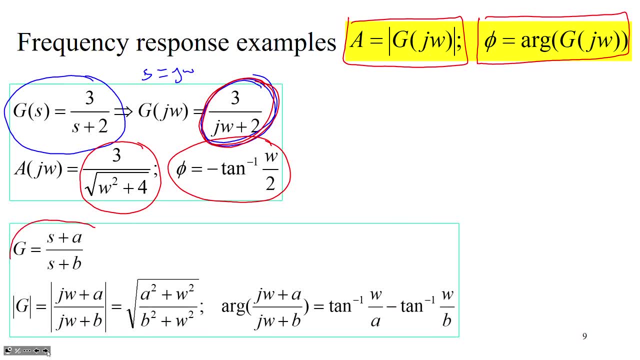 So here's a slightly more complicated example. I've got G equals s plus a over s plus b, And again you'll see I've simply replaced the s by j omega. The gain is the modulus of j omega plus a over j omega plus b. 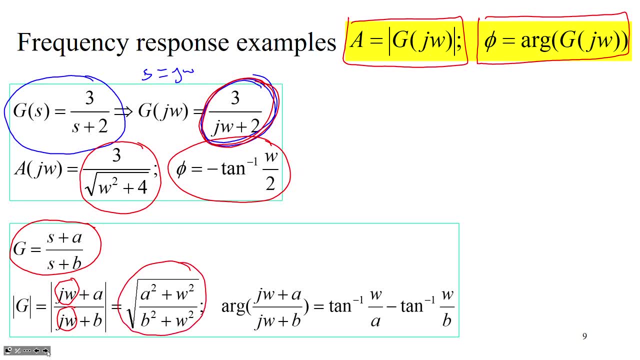 And again, assuming you're familiar with your complex numbers, you can write that by inspection using Pythagoras. And similarly, if you want the argument, you can see. it's the argument of the numerator minus the argument of the denominator. So here's another example which we can do slightly more slowly. 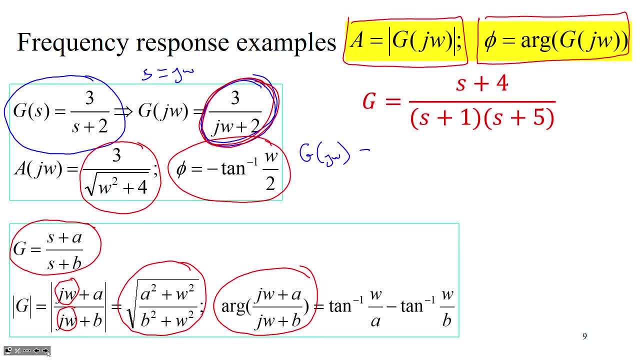 So the first thing I'm going to do is write G of j omega, which is going to be j omega plus four, Over j omega plus one times j omega plus five. Now, if I want the gain, then the gain or the modulus of G of j omega. 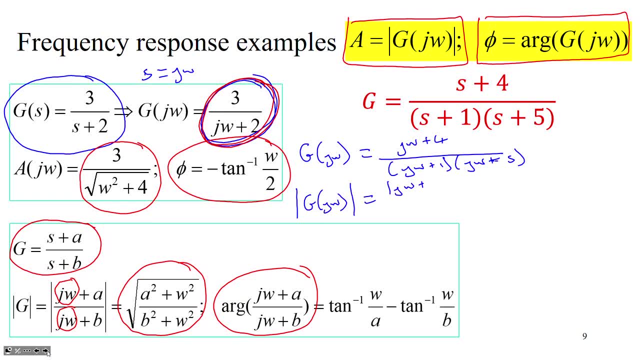 is simply going to be the modulus of j omega plus four divided by the modulus of j omega plus one times the modulus of j omega plus five And hopefully you can see by inspection that's the square root of omega squared plus sixteen over the square root of omega squared plus one. 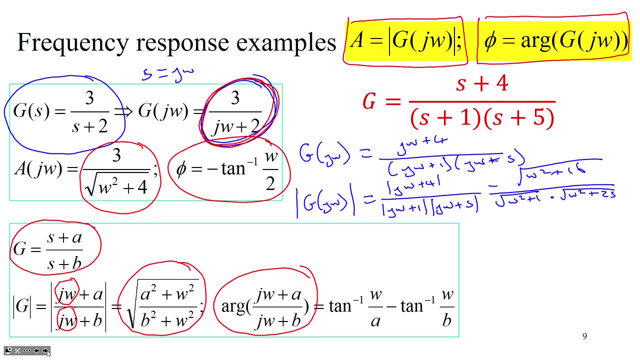 times the square root of omega squared plus twenty-five. And hopefully you see, yes, it's straightforward, And if I want the phase, so the argument of G of j omega is simply going to be the argument of j omega plus four, minus the argument of j omega plus one. 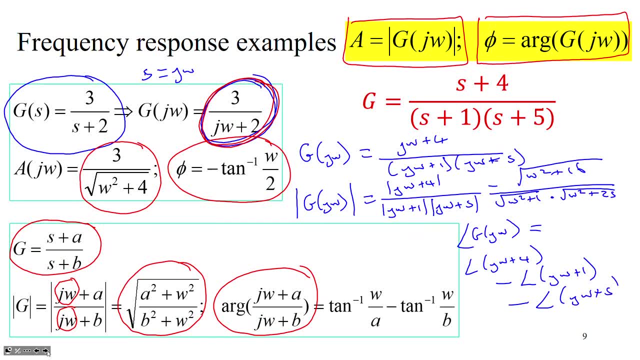 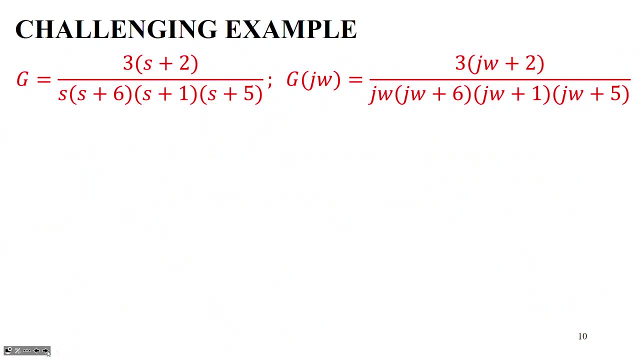 minus the argument of j, omega plus five, And you can do each of those using an inverse tan. This is a slightly more challenging example And this is just to basically say: do you know your complex numbers? And what you should know is the modulus of a, b, c. 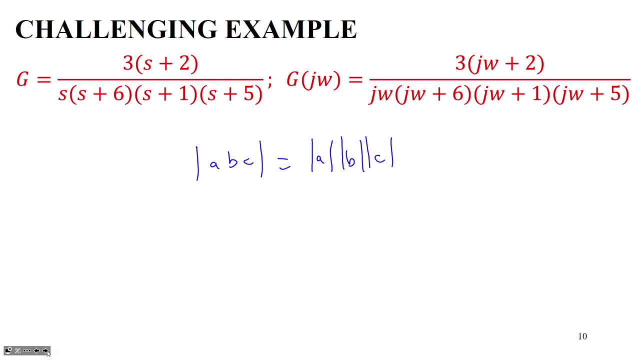 is simply the modulus of a times the modulus of b, times the modulus of c, And the argument of a, b, c is the argument of a plus the argument of b plus the argument of c. So if you know your complex numbers, you can see I can split this seemingly complicated function. 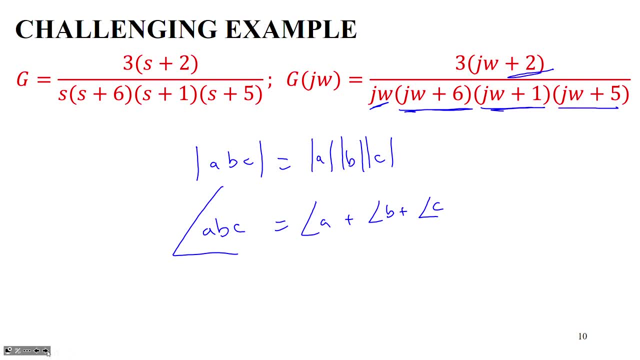 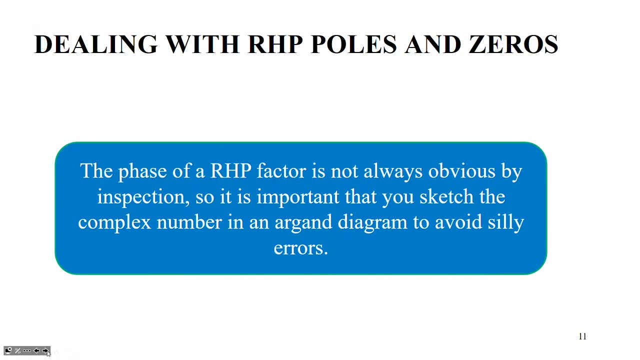 into five different groups. I can split complex numbers and just use the product rule and the addition rule with the arguments. What happens then if I have right half plane poles and zeros? Well, the phase of a right half plane factor is not always obvious by inspection. 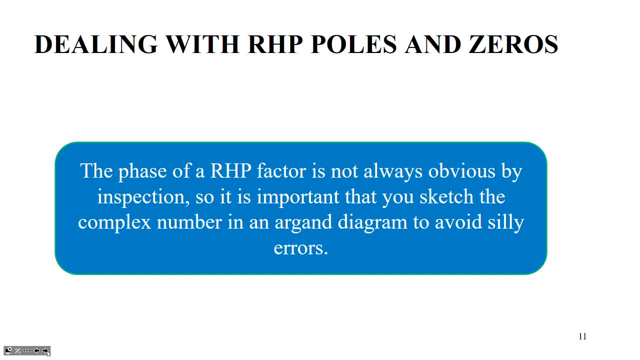 And so this is my recommendation: You don't have to do it, but it will help you avoid mistakes. If you have a right half plane factor, always do a sketch just to make sure you don't make a silly error. So here's an example. 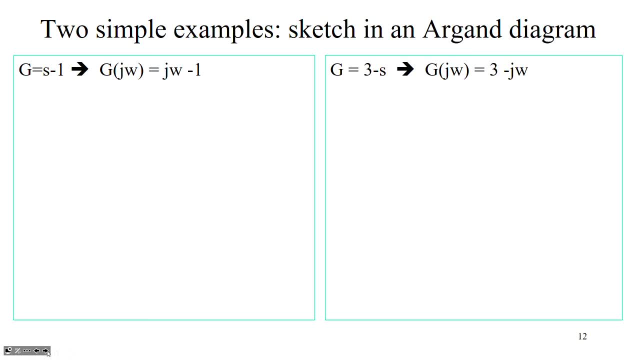 I've got g equals s minus one, or g of j omega is j omega minus one. And what I'm going to do is I'm going to do a sketch- Here's my diagram- with real and imaginary, And I'm going to put this complex number. 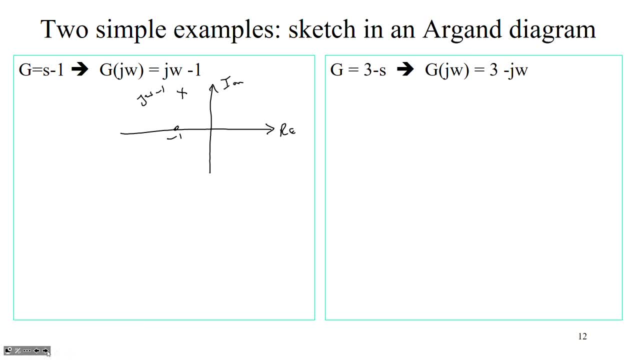 There it is j omega minus one, And the key thing is I can see the phase is theta And I can see which quadrant it's in. So if I want to get the phase, I can avoid silly mistakes by making sure I can see this Argand diagram. 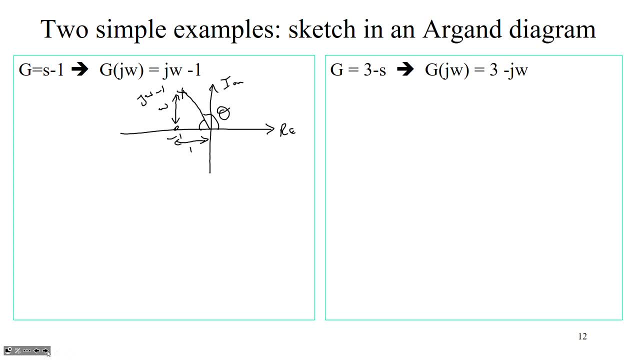 So there's omega and there's one, So I can calculate phi And what I can see is that theta equals 180 minus phi, which is 180 minus tan, to the minus one of omega over one. So you see, by plotting the Argand diagram, 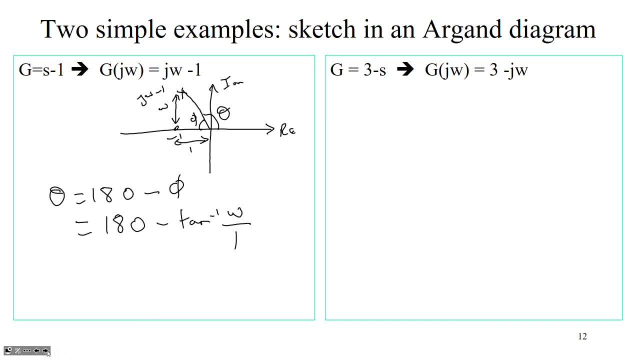 I can make sure I don't make any silly mistakes calculating the phase. Similarly, for this second example, I've got three minus j omega, So there's three. Here's the point: three minus j omega. So this distance is omega. This distance is three. 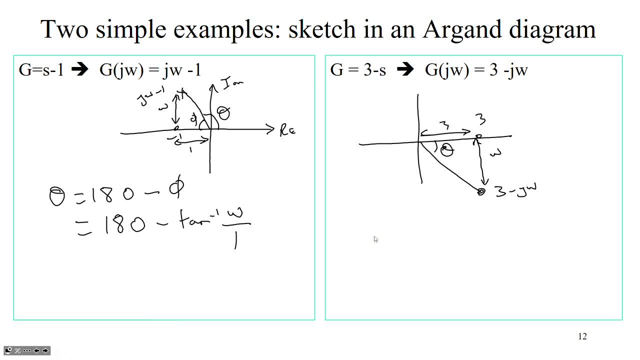 And there's my Argand theta. So theta, oops, I don't know what happened there. Theta is clearly tan to the minus one, Sorry, minus tan to the minus one Of omega over three. Now you notice I've got a very different formula here, haven't I? 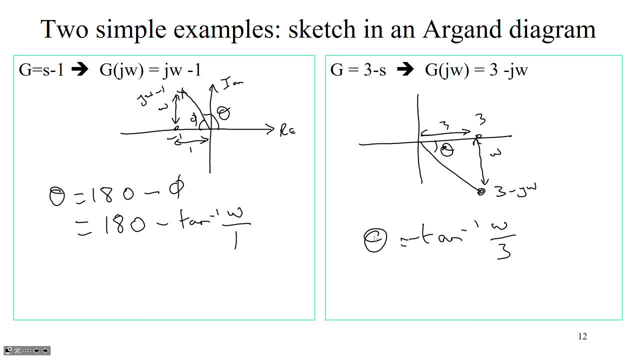 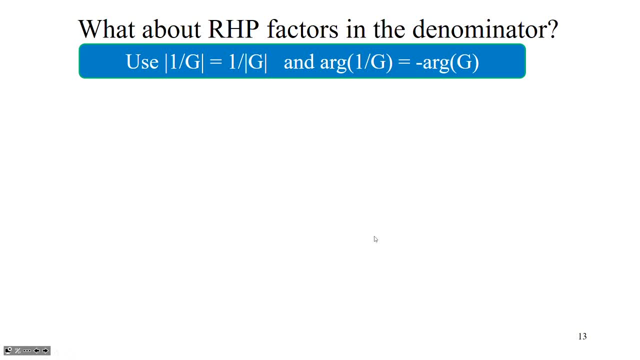 for these two complex numbers. One's got 180 in it and the other doesn't. What happens if I have a right half-plane factor in the denominator? Well, this: you just need to remember again your complex number algebra, that the modulus of one over g is the same as one over the modulus of g. 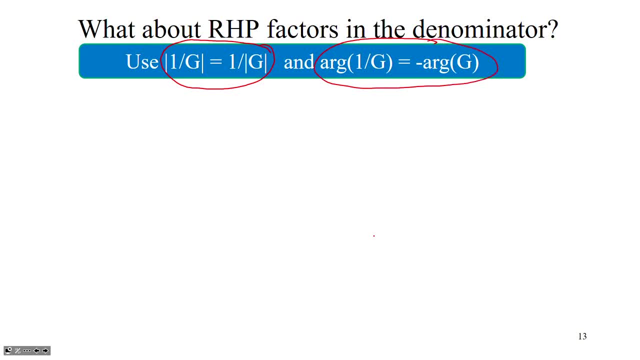 And the argument of one over g is the same as minus the argument of one over g. So if I have one over s minus one, what I'm going to do is I'm going to go back quickly And I'm going to see I've already done j omega minus one. 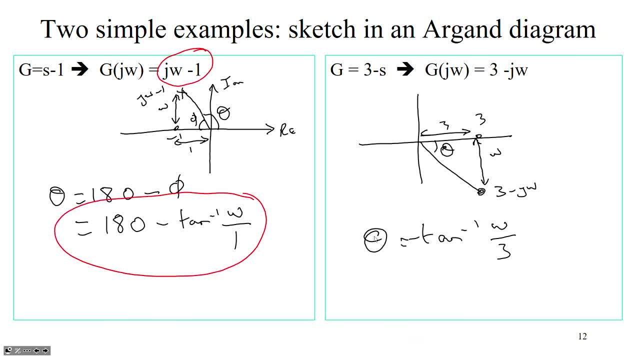 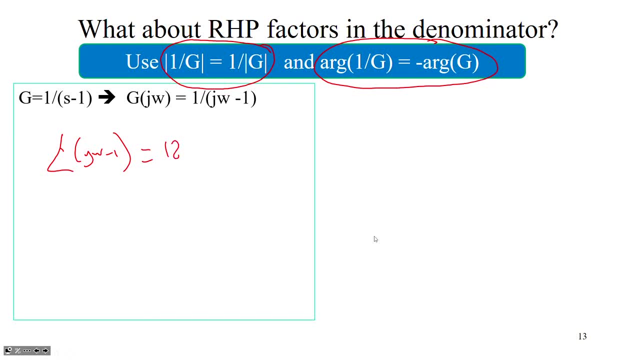 Here it is, So let's write that down first. OK, So the argument of j omega minus one equals 180 minus tan to the minus one of omega over one, So that I did on the previous page, And therefore the argument of one over g. 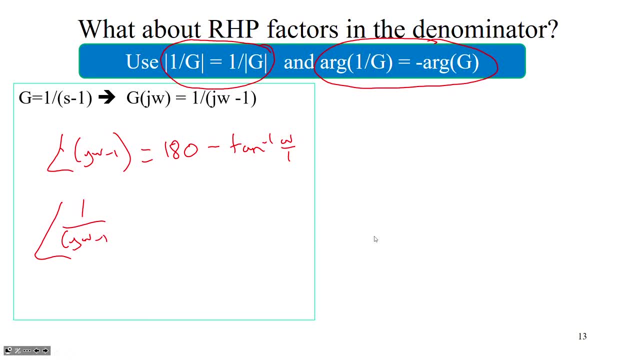 the argument of one over j. omega minus one is going to be minus 180 plus tan to the minus one of omega over one. So that's the easiest way to do that And similarly for this example here we did on the previous page that the argument of three minus j omega. 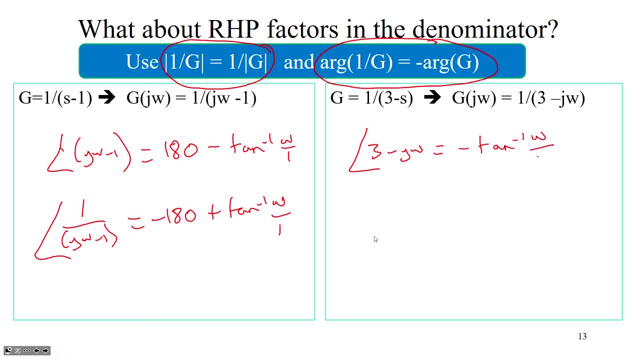 is minus tan to the minus one of omega over three And therefore the argument of one over three minus j, omega must be plus tan to the minus one of omega over three. I'm not doing the modulus, because the modulus is a lot more straightforward just using Pythagoras. 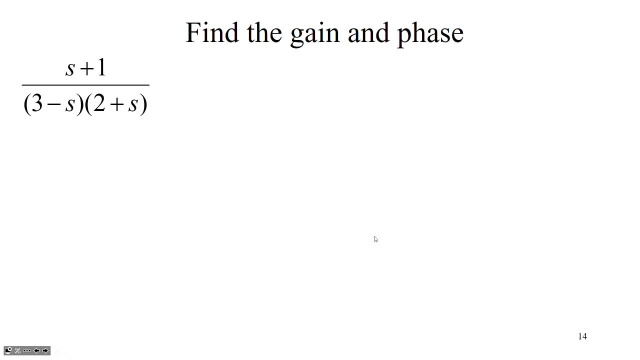 So here's an example. How would you find the gain and phase of this? So the first thing I would do is I would say the modulus of s plus one over. I better put j omega to make it clear over. three minus j omega, two plus j omega. 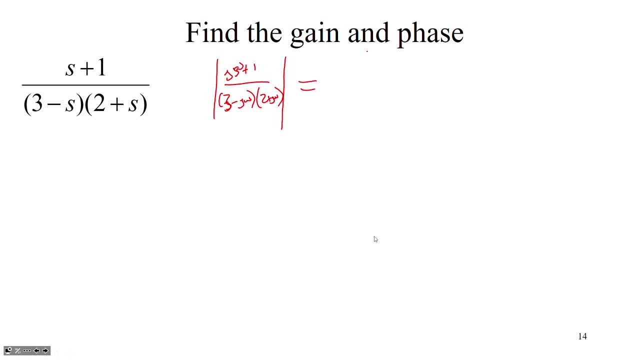 So I made that too tight, didn't I? It's going to be the modulus of j omega plus one, divided by the modulus of three minus j omega, times two plus j omega. So for the gain, I simply split it into the different factors. 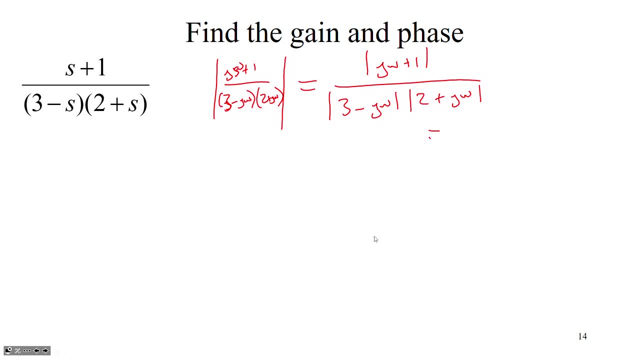 and multiply the modulus of each And hopefully you can see by inspection- you're going to get the square root of omega squared plus one divided by the square root of nine plus omega squared times two. So that becomes four plus omega squared. So the modulus is relatively straightforward with these simple factors. 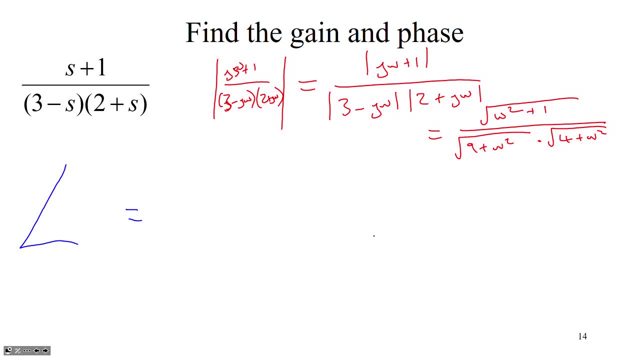 What about the phase? Well, the phase of this is going to be the phase of s plus one minus, the phase of three minus s minus the phase of two plus s. So you see how I simplify it. first I say what are my factors. 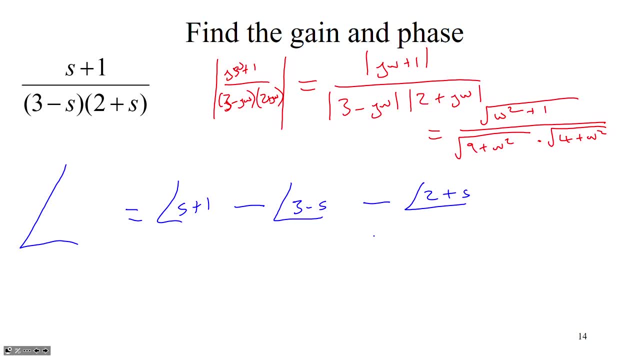 Are the factors in the denominator, in which case I have a plus, or in the denominator, in which case I put a minus. And it's as simple as that, because now you can simply write the answers down by inspection. So I get tan to the minus, one of omega minus. 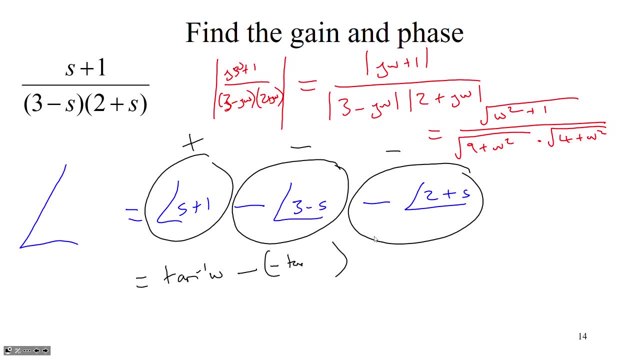 and then what was the three minus s? It was minus tan to the minus one of omega over three. We did that on the previous page- And then minus tan to the minus one omega over two. Now you'll notice how I've been careful here. 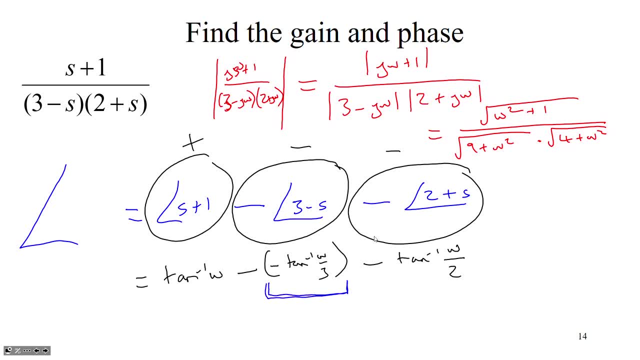 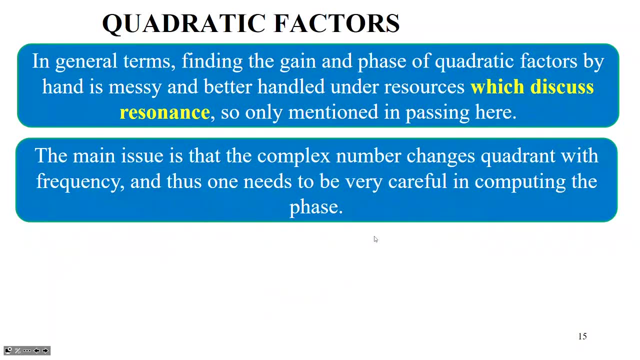 to put brackets in this expression to make sure I get all my pluses and minuses and don't get things mixed up. What about quadratic factors then? In general terms, finding the gain and phase of quadratic factors by hand is messy and I wouldn't tend to do this here. 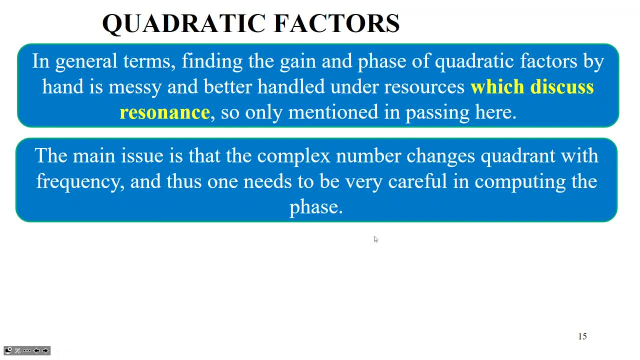 so I'm only going to mention it very, very quickly so you recognise it's messy and realise that's a topic in itself, but it's best covered when you study resonance And the big issue that you really have to worry about is the complex number changes quadrant. 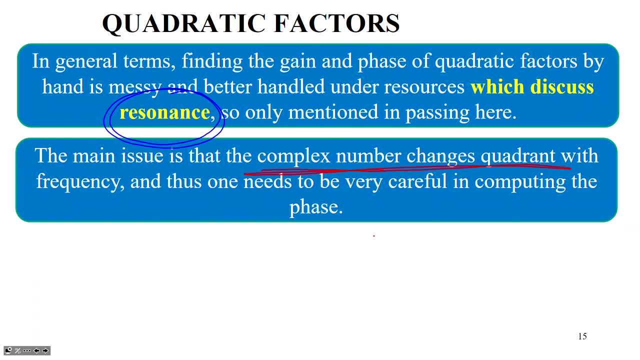 as you change frequency, So the formula you need to use changes. so that's where you have to be very, very careful. So we'll give a simple example and then leave it at that. So here's a quadratic factor s plus one, squared plus four. 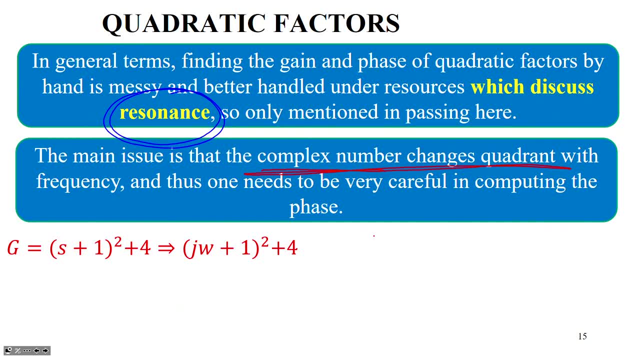 which you can write as j omega plus one squared plus four. Now the first thing I'm going to do is expand that out and you see what do I get? I get five minus omega squared plus two j omega. So the real part is five minus omega squared. 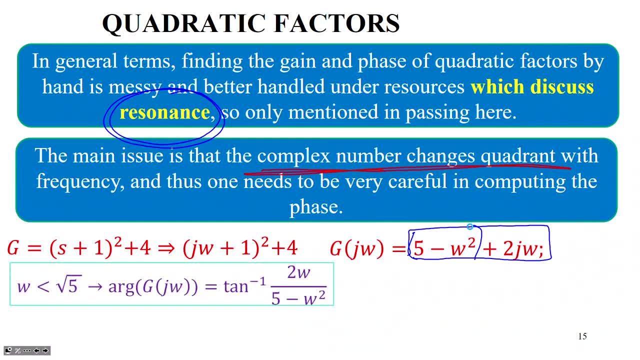 and the imaginary part two, j, omega. So what happens then if omega is less than the square root of five? And what you find is: this real part is positive. So if omega is less than the square root of five, the real part is positive.